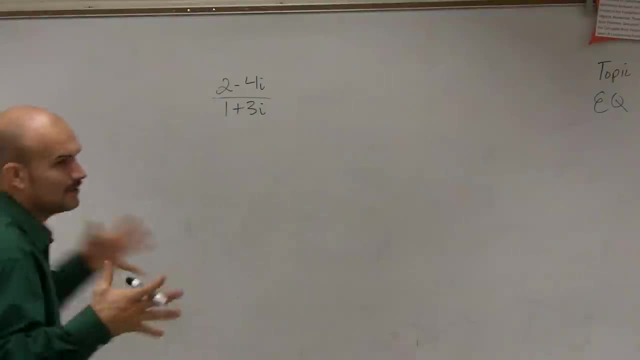 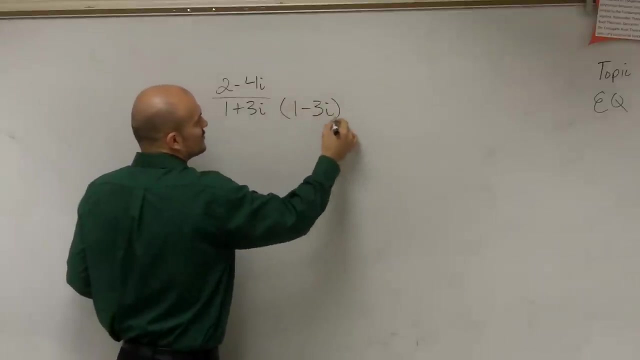 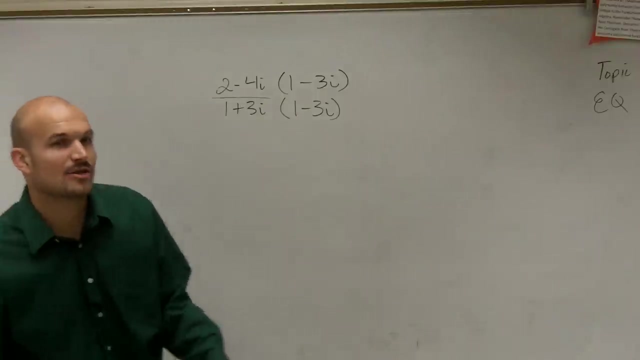 Alright. So, ladies and gentlemen, if we have 2 minus 4i divided by 1 plus 3i, The main important thing that I want to do for this problem is remember: multiply by my conjugate. So I need to make sure I understand what is my conjugate. My conjugate is 1 minus 3i. Alright, You've got to make sure you multiply by the conjugate and you've got to make sure you multiply on the numerator and the denominator. Now, remember the reason why I multiply by the conjugate is because 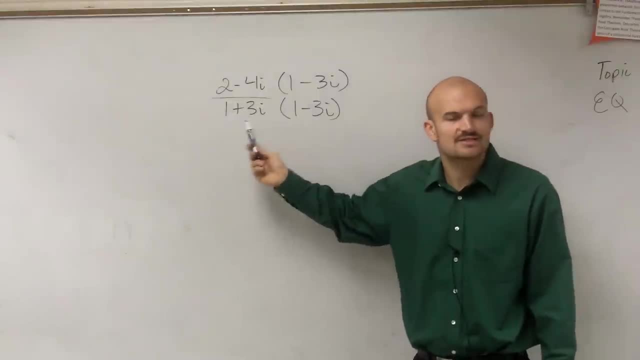 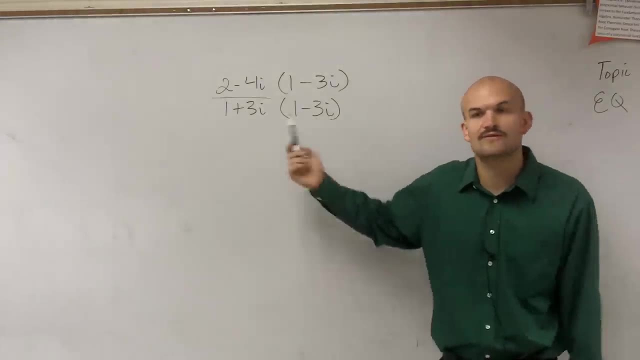 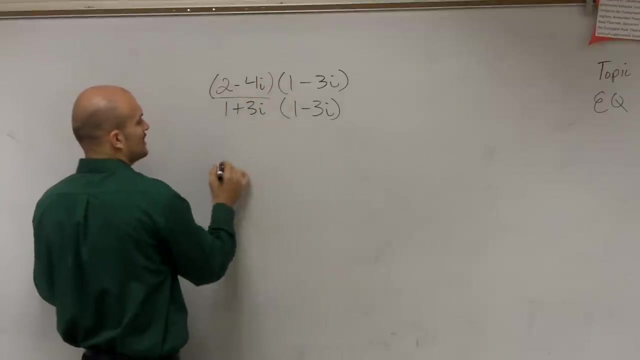 our middle terms are going to cancel out, because this is representing difference of 2 squares. and then also, I'm going to have i times i, which is going to give me i squared, which therefore I'm no longer going to have i in the denominator. So what I'm going to do is same thing: I need to multiply the top by using FOIL, So therefore I have 2 minus 6i, minus 4i, plus 12i squared. That's by multiplying. 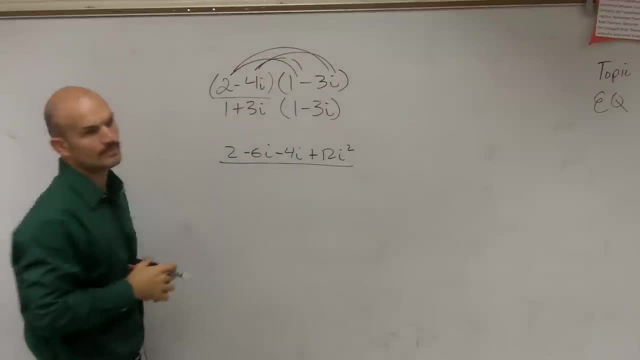 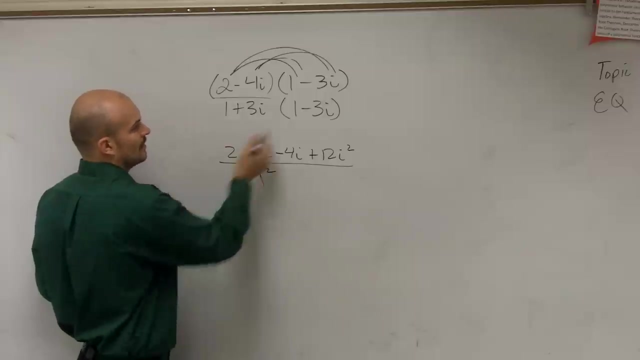 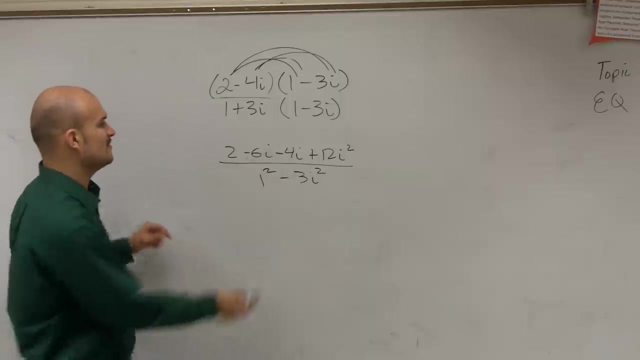 all your terms by each other, Right, Then I multiply the bottom. But on the bottom I can use- since I know I'm using difference of 2 squares- I know my middle terms are going to cancel out. Therefore, I can just rewrite the first 2 terms multiplied by each other and then I can have negative 3i squared, Because I know the middle terms already cancel out. So now to simplify this: negative 6i minus 4i is negative 10i. Then i squared is negative. 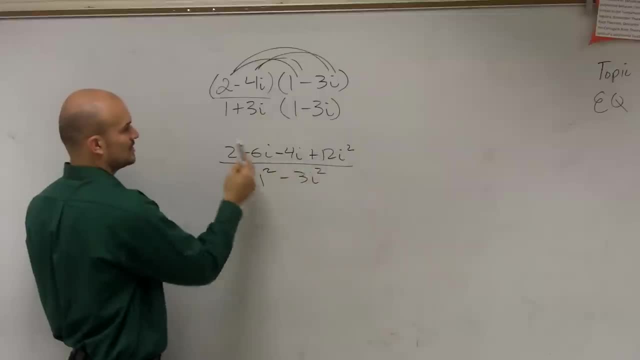 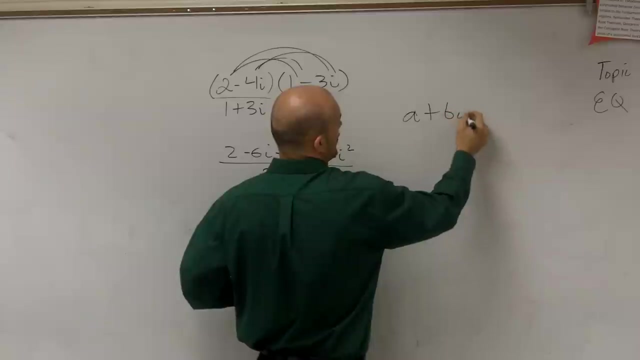 1. Negative 1 times 12 is negative. 12. Negative 12 plus 2 is negative. 10 minus 10i divided by i squared is negative. 1. Negative 1 times negative 3 is positive. 3. Positive 3 plus 1 is 4.. However, ladies and gentlemen, you remember we talked about writing complex numbers in the form of a plus bi, Not a plus bi divided by a number. Yes, 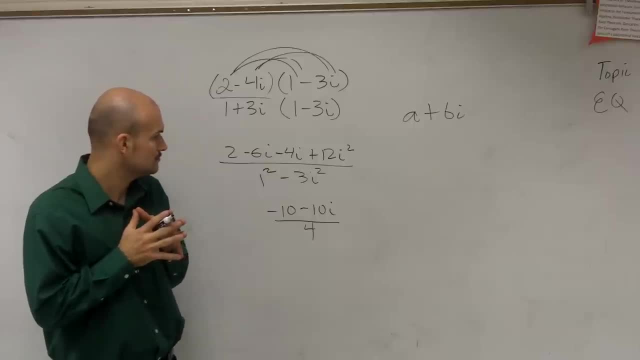 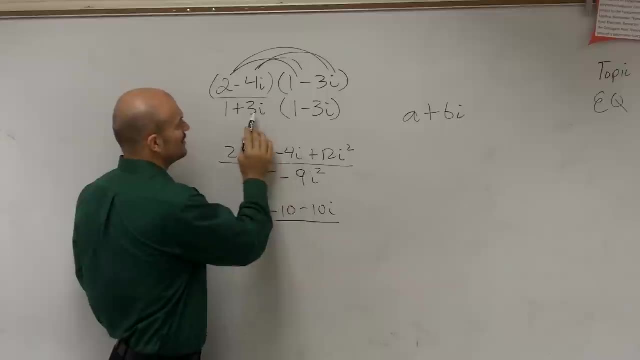 It would be 9i squared. You're right, Thank you, Thank you, Thank you. 3i times negative 3i is 9i squared, So therefore it's going to be a positive 9,, which would be a- I'm sorry- positive 9,. right, So it would actually be 10.. Thank you very much. Thank you. 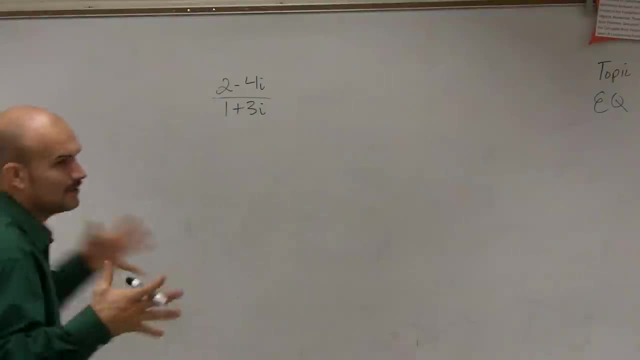 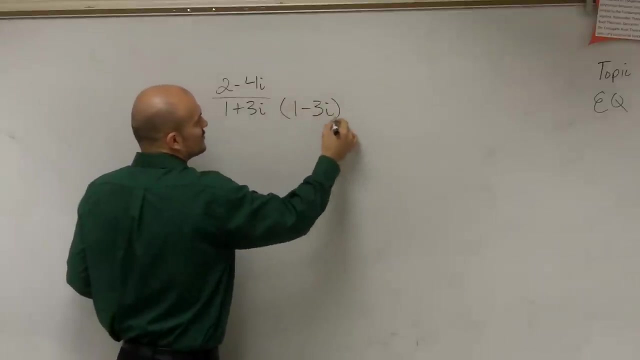 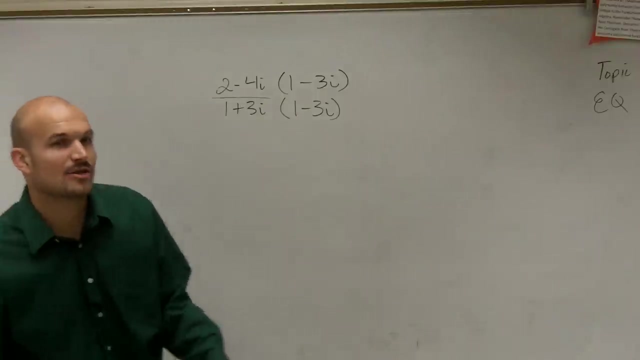 Alright. So, ladies and gentlemen, if we have 2 minus 4i divided by 1 plus 3i, The main important thing that I want to do for this problem is remember: multiply by my conjugate. So I need to make sure I understand what is my conjugate. My conjugate is 1 minus 3i. Alright, You've got to make sure you multiply by the conjugate and you've got to make sure you multiply on the numerator and the denominator. Now, remember the reason why I multiply by the conjugate is because 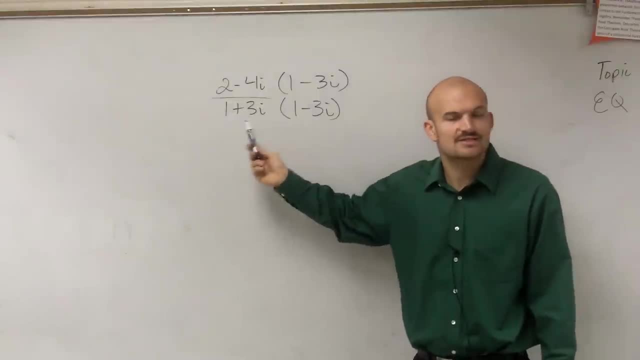 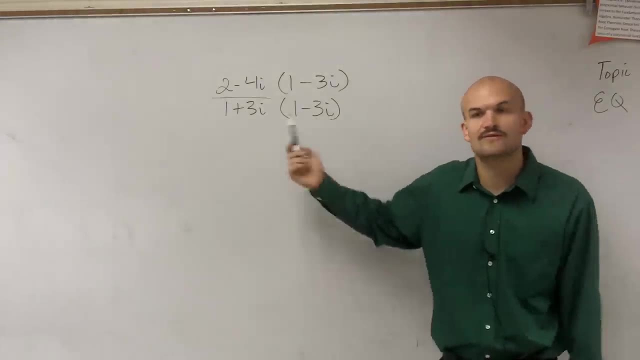 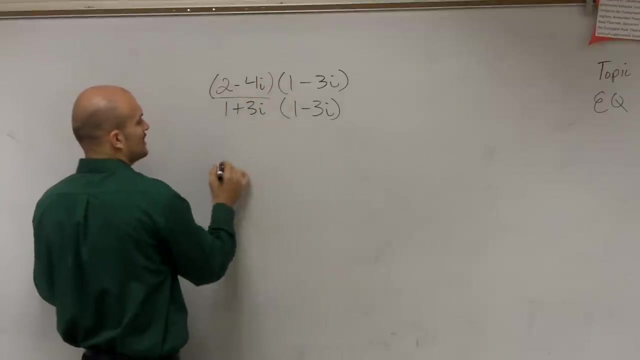 our middle terms are going to cancel out, because this is representing difference of 2 squares. and then also, I'm going to have i times i, which is going to give me i squared, which therefore I'm no longer going to have i in the denominator. So what I'm going to do is same thing: I need to multiply the top by using FOIL, So therefore I have 2 minus 6i, minus 4i, plus 12i squared. That's by multiplying. 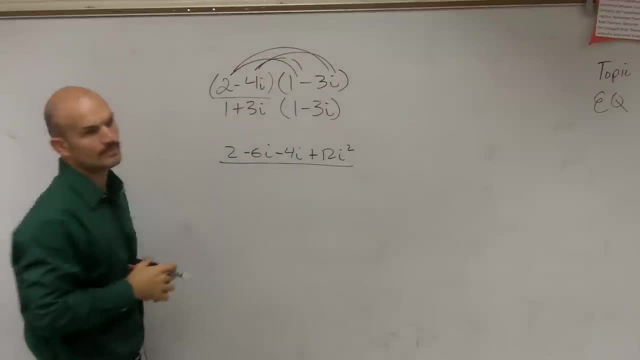 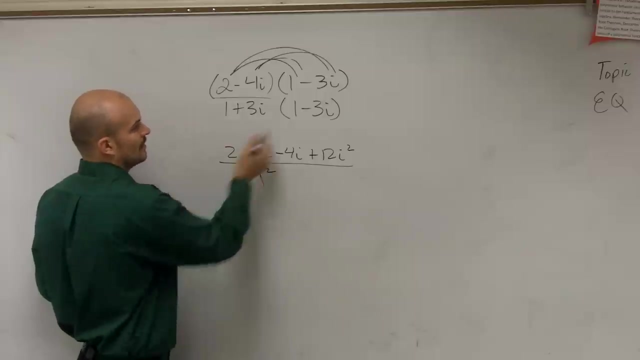 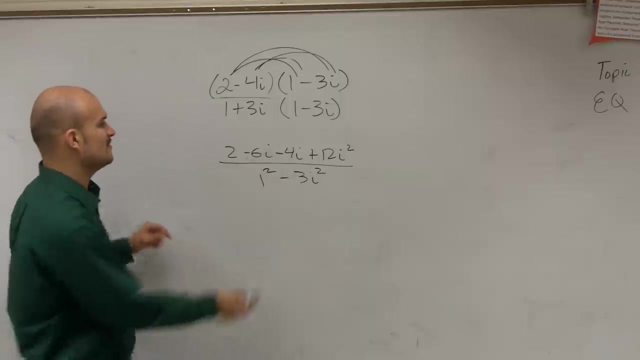 all your terms by each other, Right, Then I multiply the bottom. But on the bottom I can use- since I know I'm using difference of 2 squares- I know my middle terms are going to cancel out. Therefore, I can just rewrite the first 2 terms multiplied by each other and then I can have negative 3i squared, Because I know the middle terms already cancel out. So now to simplify this: negative 6i minus 4i is negative 10i. Then i squared is negative. 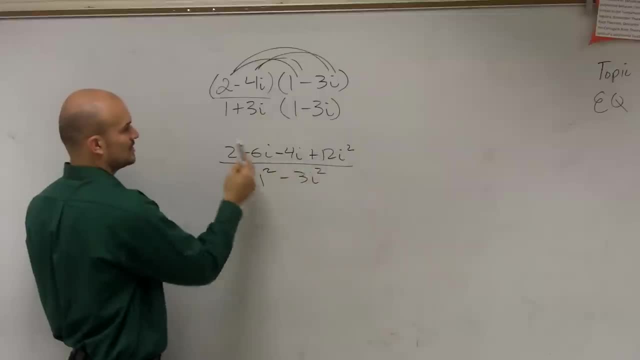 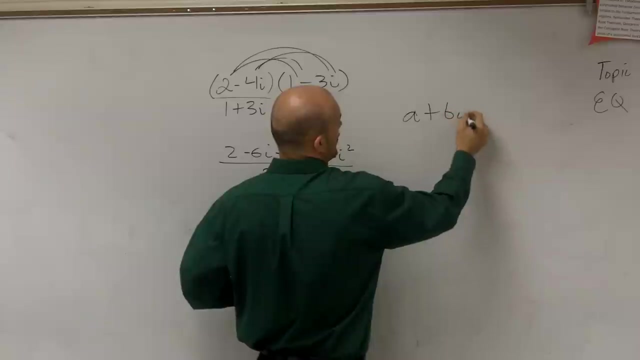 1. Negative 1 times 12 is negative. 12. Negative 12 plus 2 is negative. 10 minus 10i divided by i squared is negative. 1. Negative 1 times negative 3 is positive. 3. Positive 3 plus 1 is 4.. However, ladies and gentlemen, you remember we talked about writing complex numbers in the form of a plus bi, Not a plus bi divided by a number. Yes, 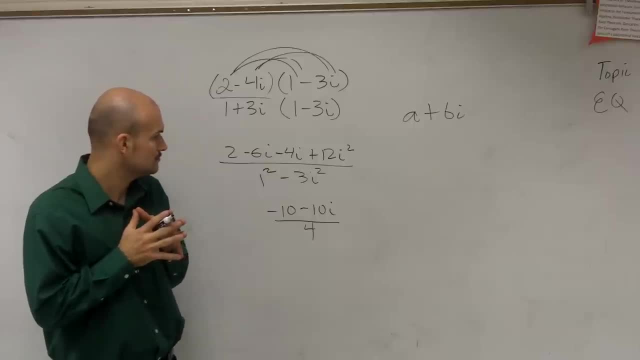 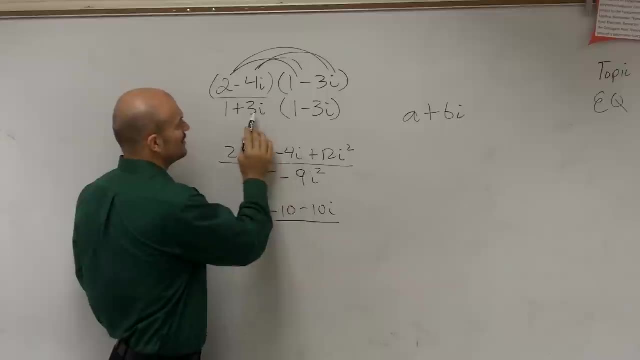 It would be 9i squared. You're right, Thank you, Thank you, Thank you. 3i times negative 3i is 9i squared, So therefore it's going to be a positive 9,, which would be a- I'm sorry- positive 9,. right, So it would actually be 10.. Thank you very much. Thank you.